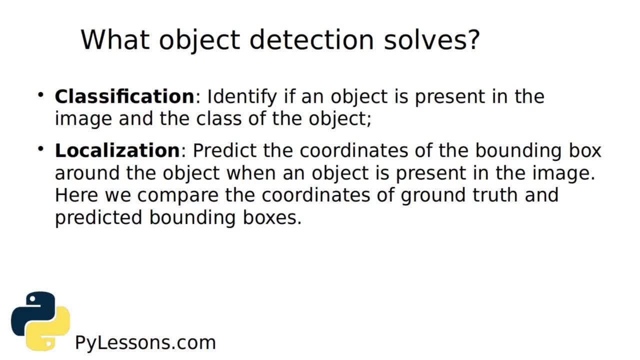 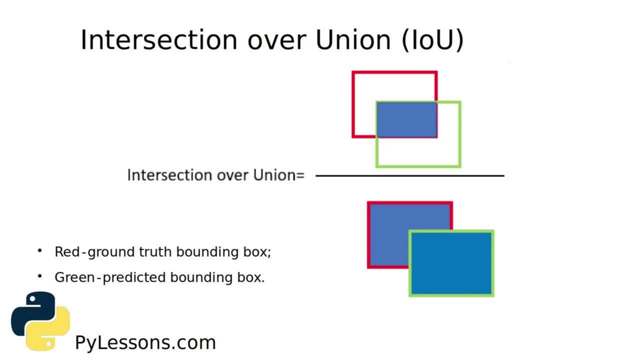 as well as the localization of using bounding box boxes in the image. For object detection we use the concept of intersection over union. This means that we are measuring overlap between two boundaries. So actually we use that to measure how much our predicted boundary overlaps with the. 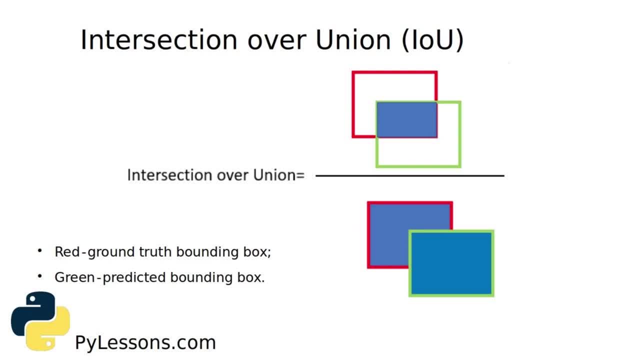 ground truth bounding box. The ground truth is the real object boundary Here. in this slide you can see that ground bounding box is ground truth and grid bounding box is predicted box. In simple terms, intersection over union tells us how well predicted and ground truth bounding box overlap You. 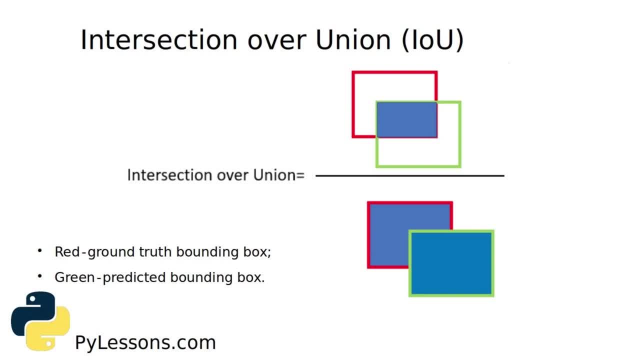 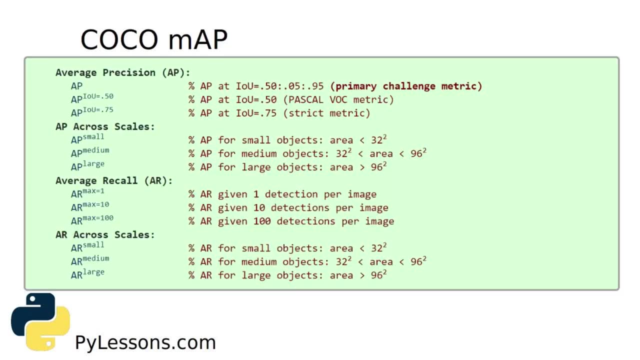 will see that in my code we can set a threshold value for IOU to determine if the object detection is valid or not. So, for example, for Coco, AP is the average over multiple intersection over unions. This means that the minimum IOU is considered a positive match. Actually, in Coco the AP means 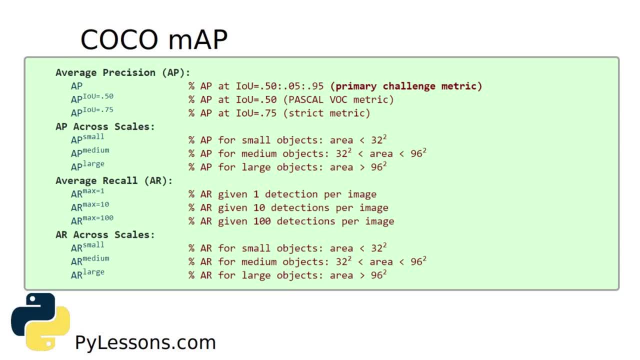 that AP corresponds to the average intersection over union in range from 0.5 to 0.95 with step size of 0.05.. For Coco implementation AP is average over 10 IOU levels in 80 categories. As I said, it starts from. 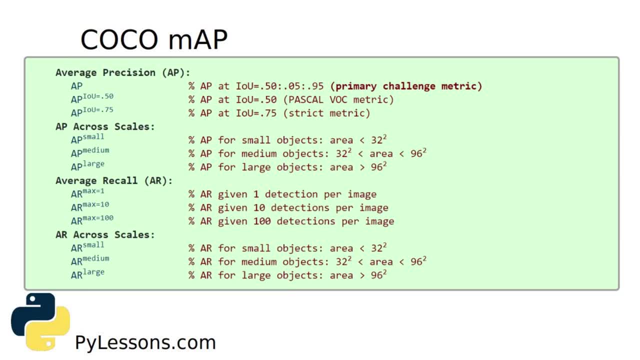 0.5 and ends at 0.95, with a step size of 0.05. and here are some other metrics collected from the coco dataset and here is the image you can see and for more information you can read on a link- and i'll post this to my text version tutorial and because my tutorial series is related to 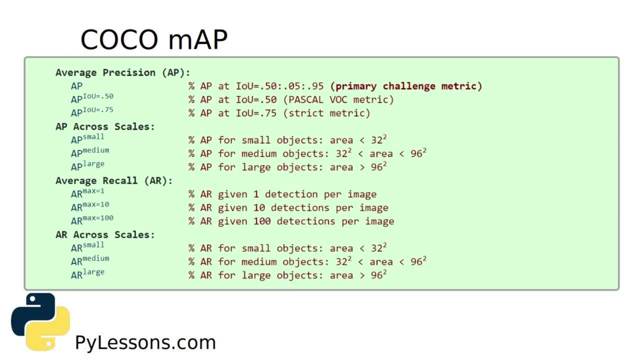 yolo v3 object detector. here we can see the results from yolo v3 paper and at the end, at last line, you can see that yolo v3 and its ap, ap 50, ap 75 and ap small, medium or large and so on. 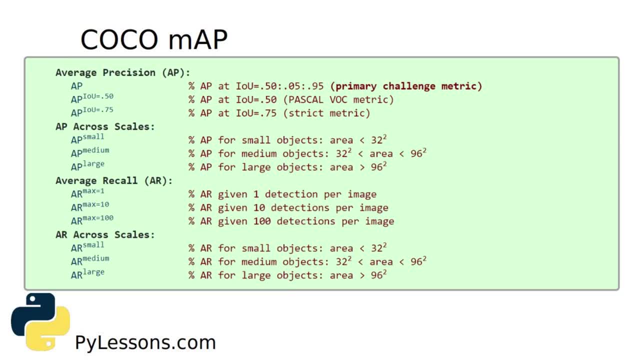 here. for example, in this figure, ap 75 means that these are results for iou 0.75 and math mean average. precision is the average of AP. in some contexts we compute the AP for each class and average them, but in some contexts they mean the same thing. 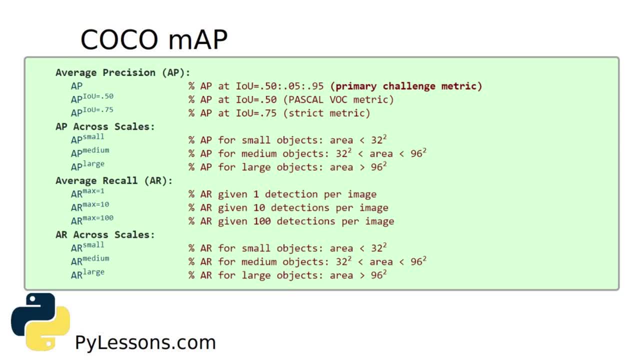 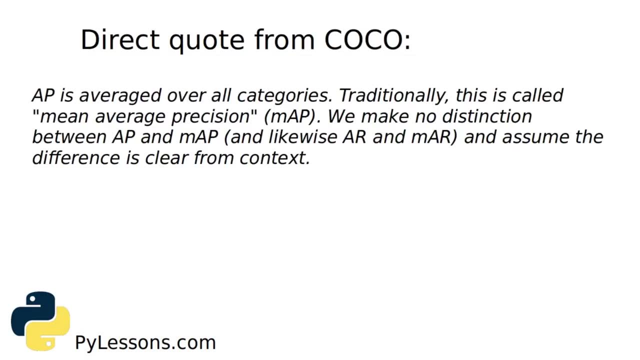 for example, under the cocoa context there is no difference between AP and map. I can quote one line from a cocoa website. so they tell that AP is averaged over all categories. traditionally this is called mean average precision. so we make no distinction between AP and map, and likewise R and MAR, and assume the difference is clear from context coming. 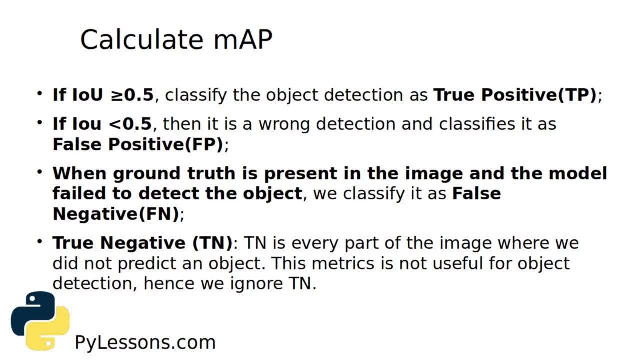 back to my tutorial. let's get back to the beginning where we need to calculate map. so first we need to set a threshold value for intersection over union to determine if the object action is valid or not. so let's say we set IOU 0.5. 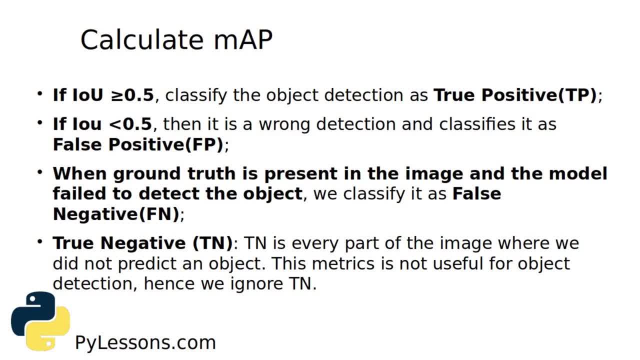 it's. this is mean that we are we are going to set the threshold value for intersection over union to determine if the object action is valid or not. so let's say we set IOU 0.5. it's this is mean that we are use a default value. if IOU is more than 0.5, we classify the object detection as 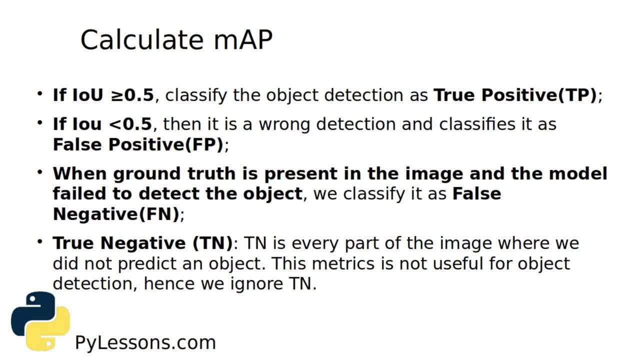 true, positive, otherwise it's wrong detection and we classify it as false positive. when ground truth is presented in the image and the model failed to detect the object, we classify it as false, negative. and the last one is true negative. true negative is every part of image where we did not predict an object. but this metric is: 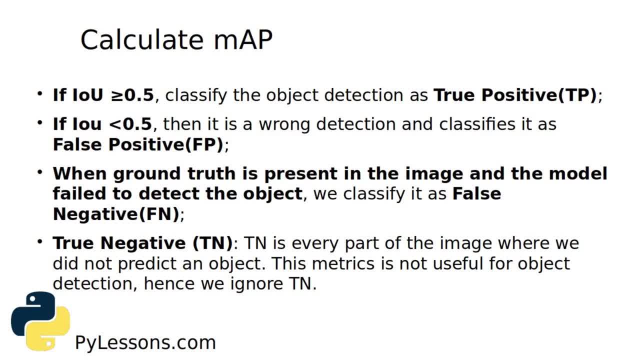 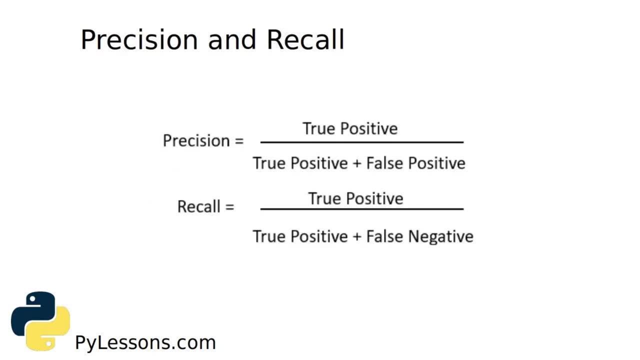 not useful for object action and we ignore it in our implementation. so if we set an IOU threshold value to 0.5, we'll calculate map 50. if we set IOU 0.75, then we'll calculate map 75. sometimes we can see this a little bit different, but 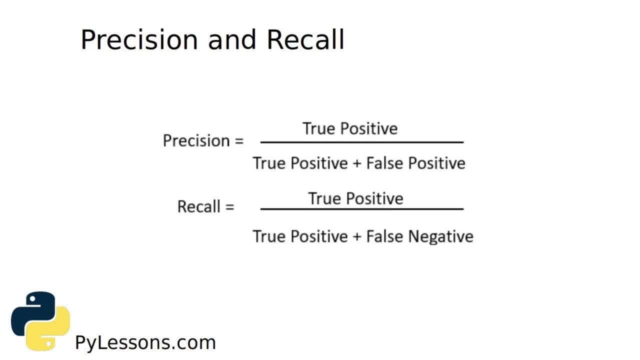 actually this is the same, so we use a precision and recall as a metric to evaluate the performance. precision and recall are calculated using true positive, false positive and false negative. as you can see from this slide, there is one difference in precision: in recall. as you can see it. 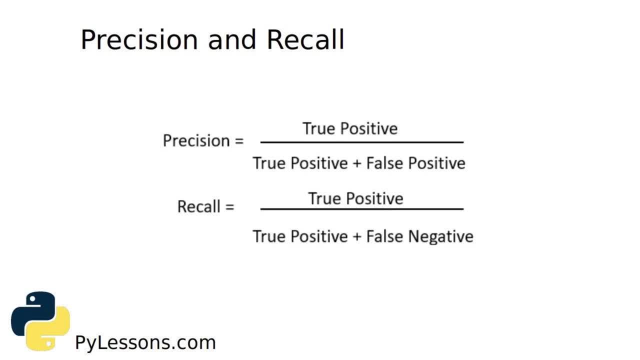 only changes from false positive to false negative. that's it. to get map, we should calculate precision and recall for all the object presented in the images. it also needs to consider the confidence score for each object detected by the model in the image model so that we can more accurately determine the performance of the object, even if it is exclude from their total gummy. 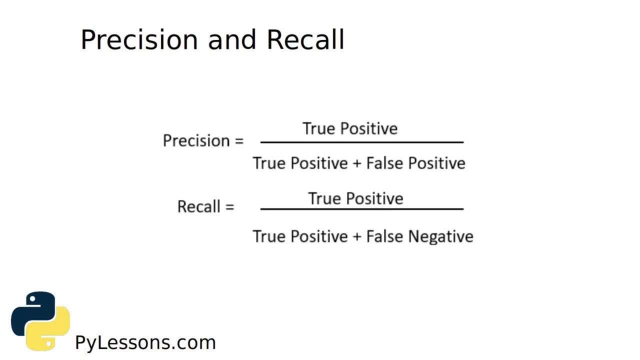 Consider all of the predicted boxes with a confidence score above a curtain threshold. Bounded boxes above their threshold value are considered as positive boxes and all predicted boxes below the threshold value are considered as negative. So the higher the confidence threshold is, the lower the map will be. 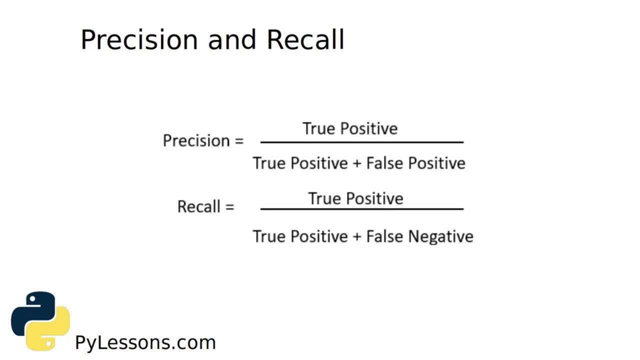 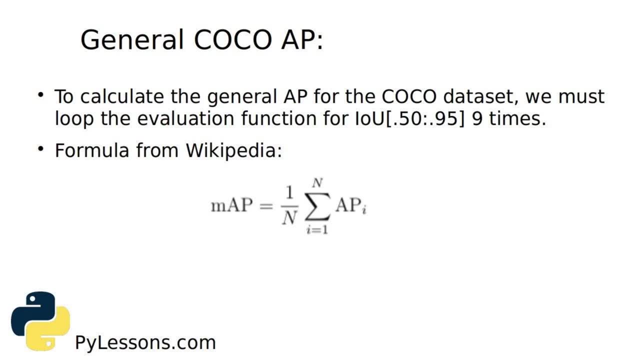 but we'll be more confident with accuracy with higher threshold. So how we actually calculate general AP? It's quite simple: For each query we can calculate corresponding AP. A user can have as many queries as he likes against his label dataset. 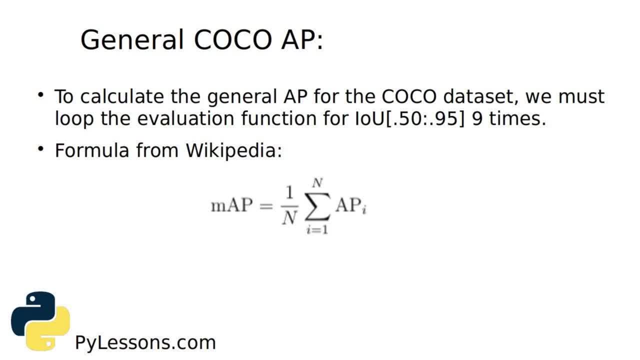 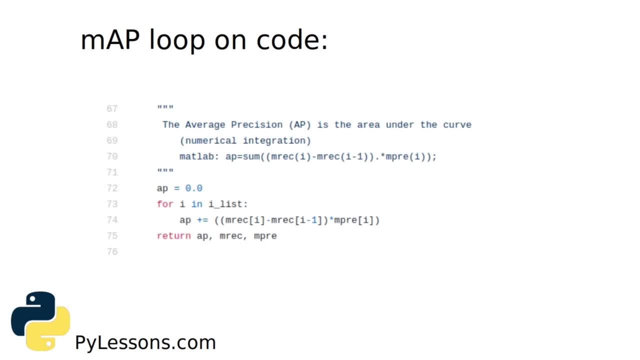 The map is simply the mean of all the queries that the user made To see how we get AP. you can check what's AP function on my GitHub repository. So when we have a precision and recall list, we simply call a simple query. 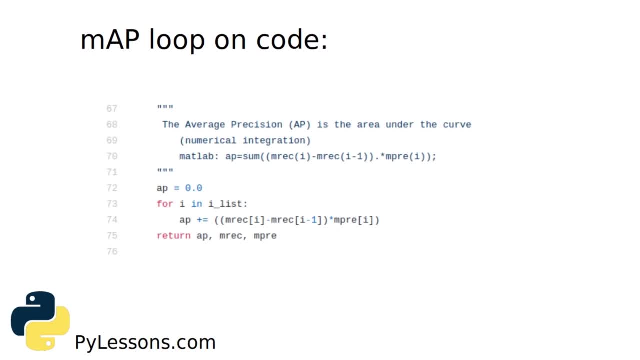 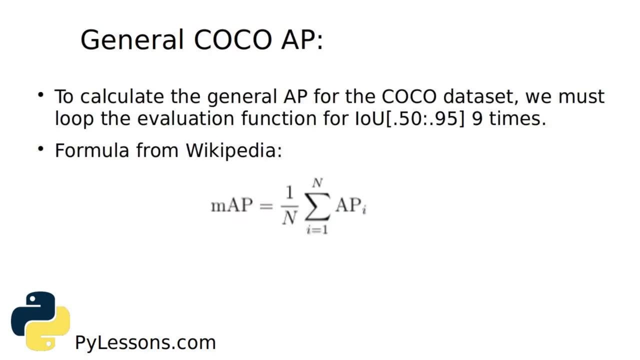 Simple loop formula And we run that formula for all classes we use. Later I will show you this formula on my GitHub repository. And to calculate the general AP for the Cocoa dataset we must loop the evaluation function for IOU nine times. Here is the formula from Wikipedia. 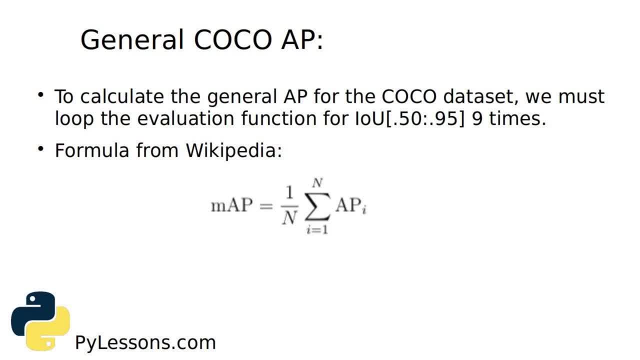 As you can see, I simply copied it, so it's quite blurry, but don't worry, It's everything right. The result is N, N will be nine and AP will be sum of all these values, from AP 50 to AP 95.. 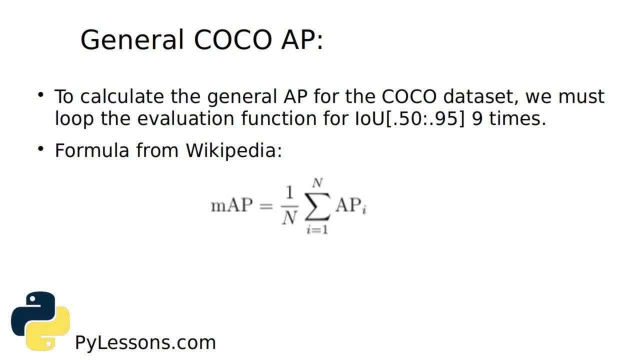 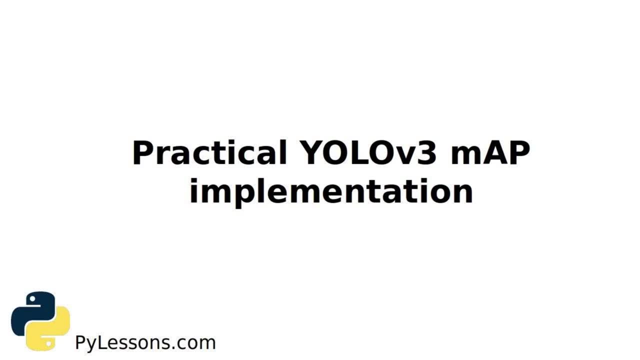 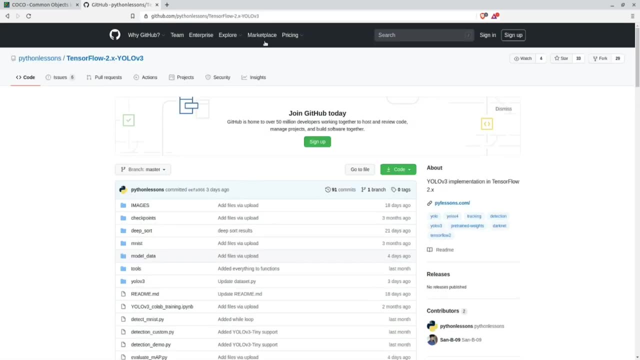 This might take a while to calculate these results, but this is the way, how we need to calculate the map. So now let's move to my practical YOLOv3 implementation. So first you should move to my YOLOv3 TensorFlow 2 implementation on GitHub. 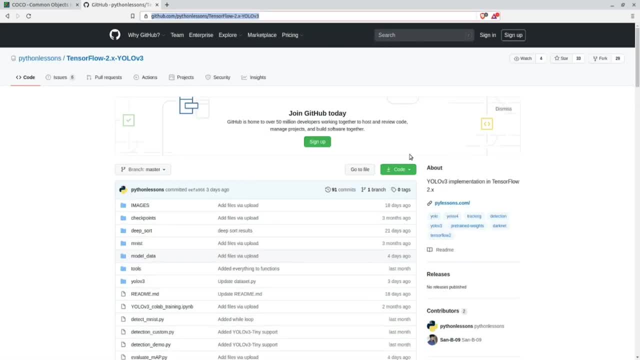 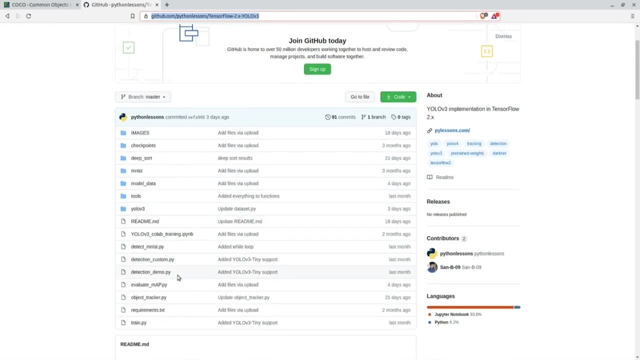 And of course I'll leave a link to my text version tour, And there is a file called YOLOv3.. It's called evaluateMap. The whole evaluation function is done in this script, So actually I can open the script. 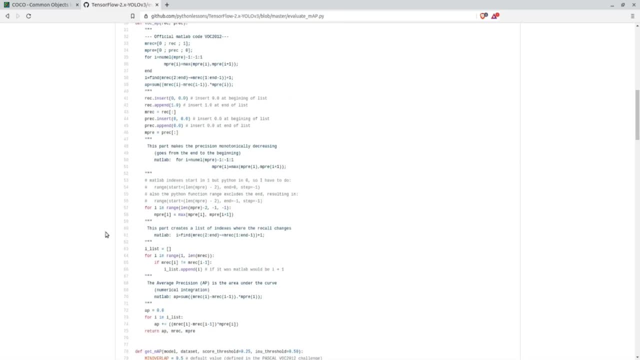 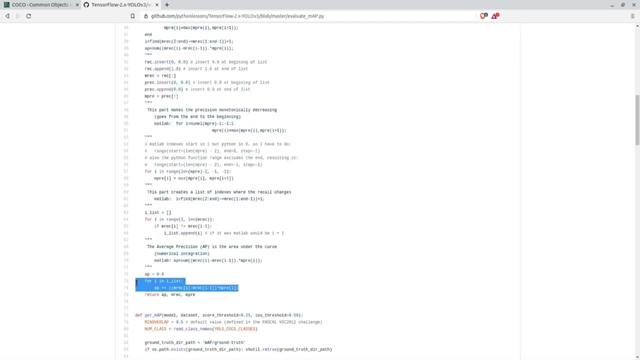 And, as I said before, we simply call one loop. So here it is For I in list. we call this and we sum all average precision metrics, We calculate, That's it. This is all. the magic happens here. 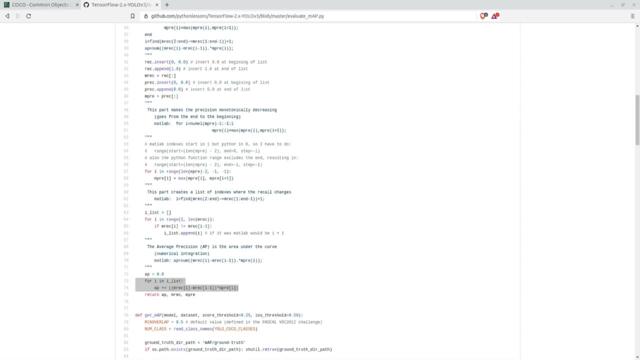 So while writing this evaluation script, I focused on the Cocoa dataset to make sure it will work on it. So in this tutorial I'll explain how to run this code to evaluate the YOLOv3 model on Cocoa dataset. So first, to reproduce my results and test everything on Cocoa dataset. 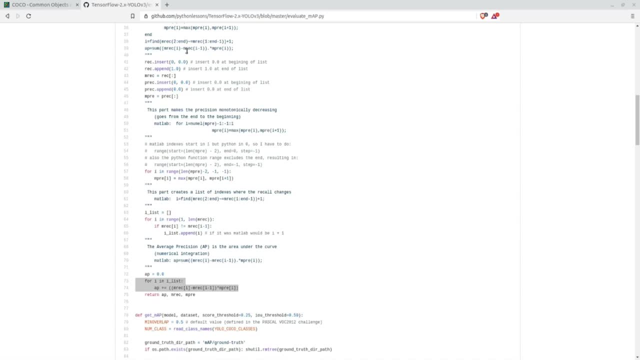 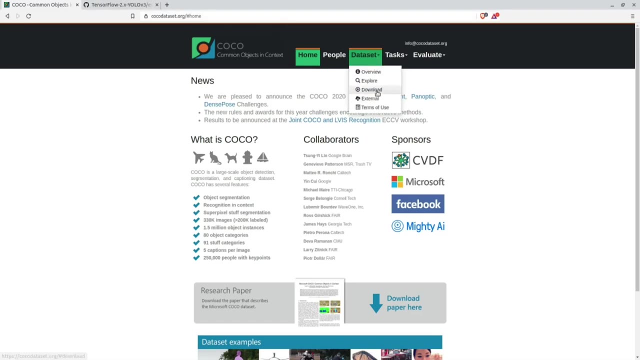 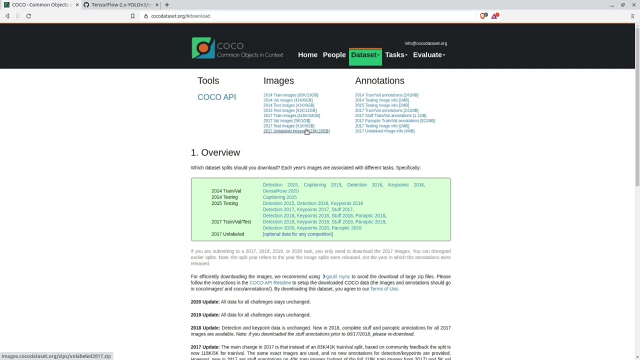 first you should download the Cocoa validation dataset from this link. I open up this cocoadatasetorg and I go to dataset downloads And there is validation images and training images. Of course, I will leave direct links to download them And, of course, you can download training files. 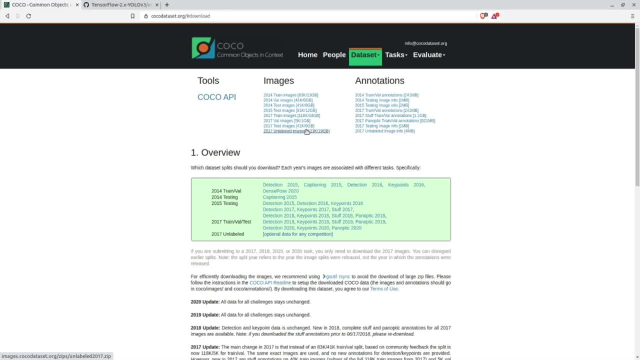 but it's not recommended. It's around 20 gigabytes of size. And, of course, why you need to train all model on Cocoa if you already have it pre-trained. So that's my strange idea for you, but it's up to you. 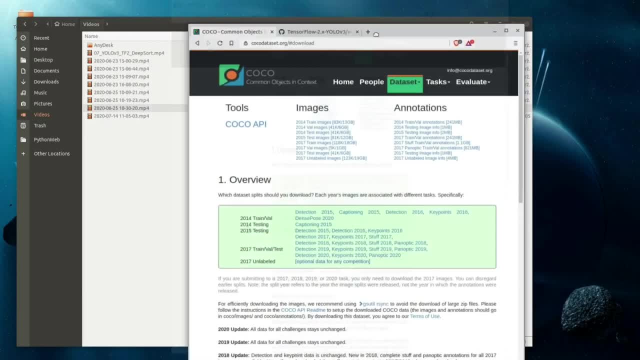 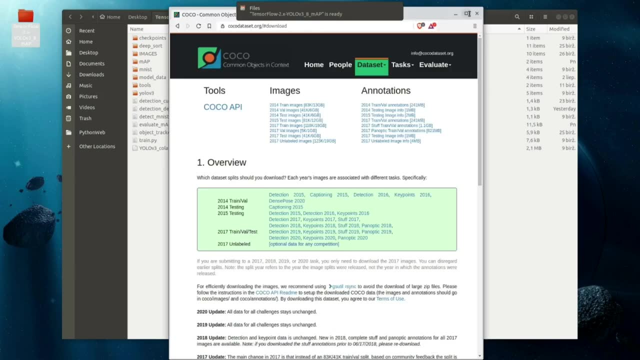 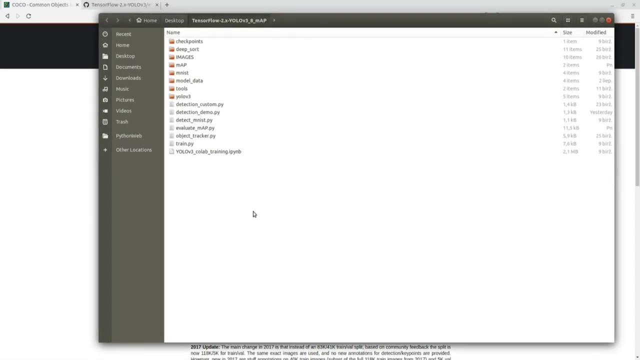 So I have here on desktop the whole repository I was working on. Okay, Here is my eighth tutorial. I have it on desktop Here. I created a Cocoa folder in model data And here is the three files, of course. 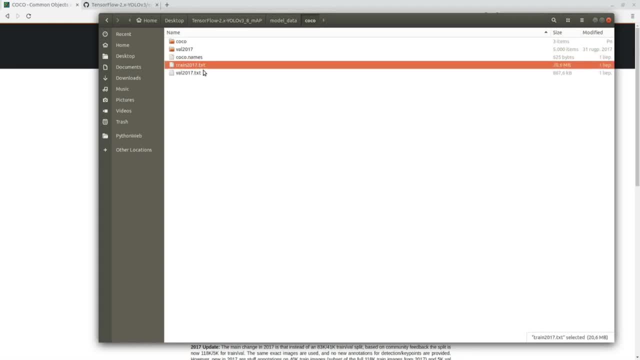 And here I created two text annotation files for you, so you don't need to worry about them. So here is validation file and here is a training file, but I won't open it because it's quite large and we don't care about that. 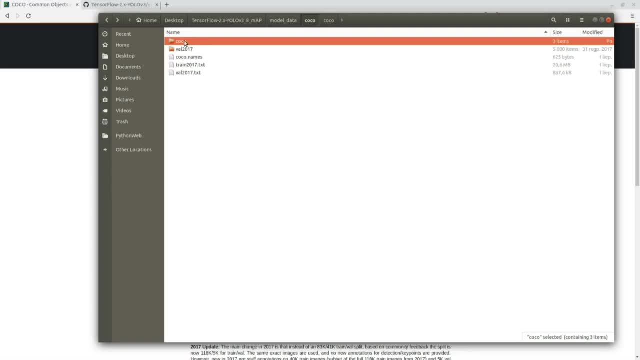 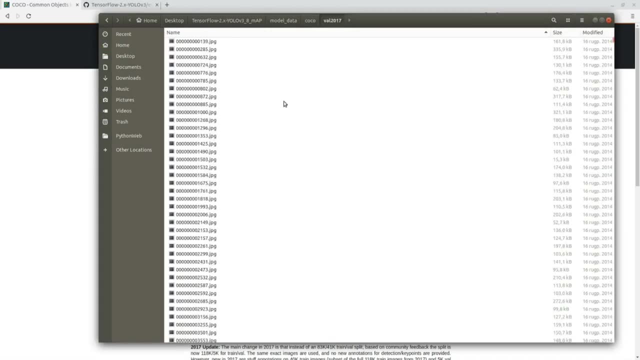 I'm not sure why there is. I think I need to remove this, but doesn't matter right now. And here is my Cocoa name And, of course, here is all the validation images from Cocoa dataset And we can see, and, as you can see, 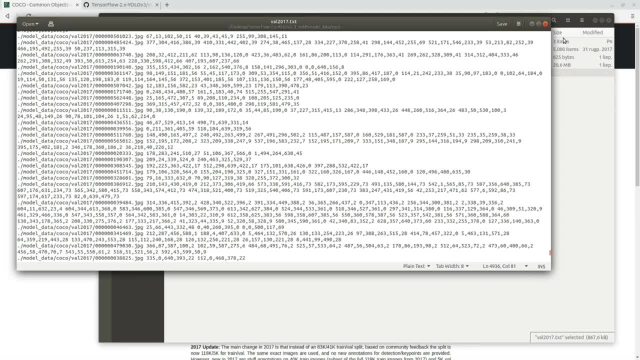 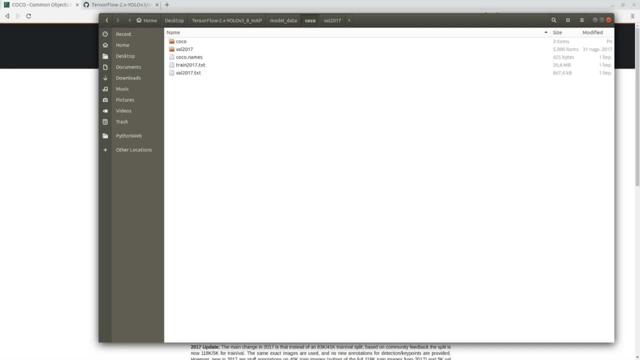 it links to this Cocoa value and image and so on. So it's everything here. You need to only download validation or training dataset. So next, if you download my repository, you will need to change the configurations file to reproduce all the results. 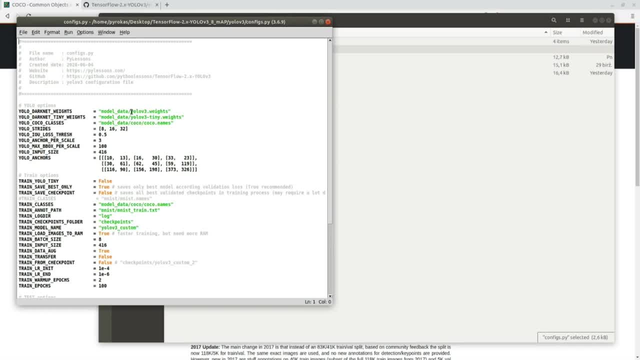 So first you need to go to your free configspy file and here is training classes line. Here was before MNIST and you need to comment this and change this to Cocoa Connect Cocoa names. of course, Here also should be Cocoa names. 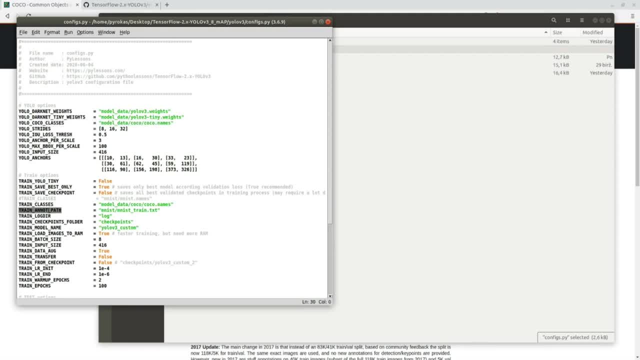 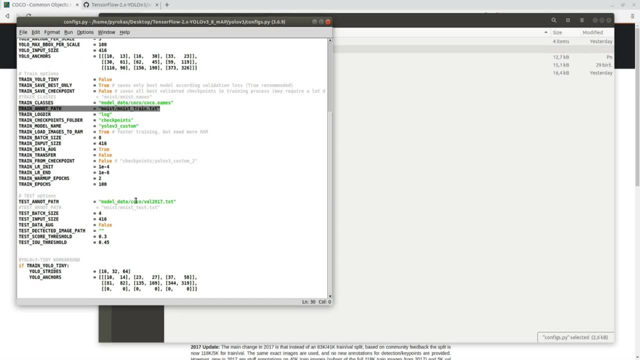 If you want to train it, of course you need to change this train annotation path. but because I'm only validating, I'm not changing this line And of course, if we would like to validate, we need to change this test annotation path. 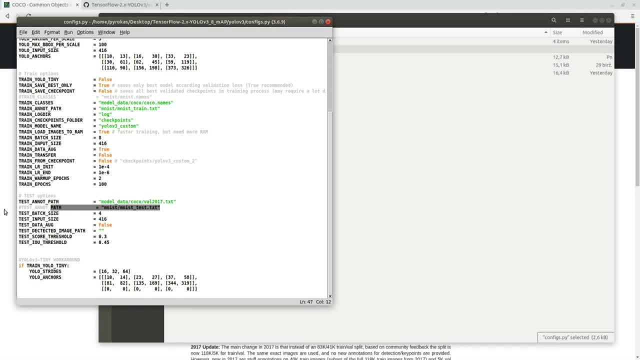 And here I just left commented, but you will need to change this by yourself. I'm not changing this, I'm just mentioning this in this video tutorial. Of course, I leave them as it was before. So now we have all settings for set for evaluation. 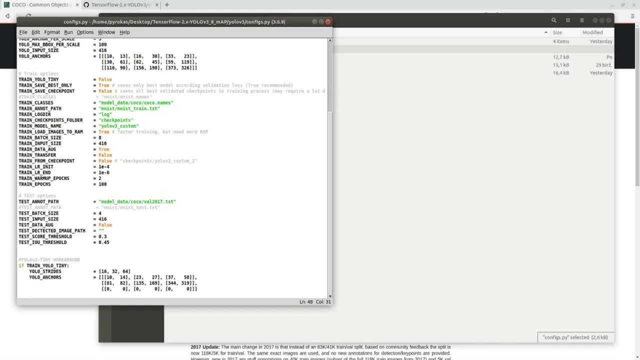 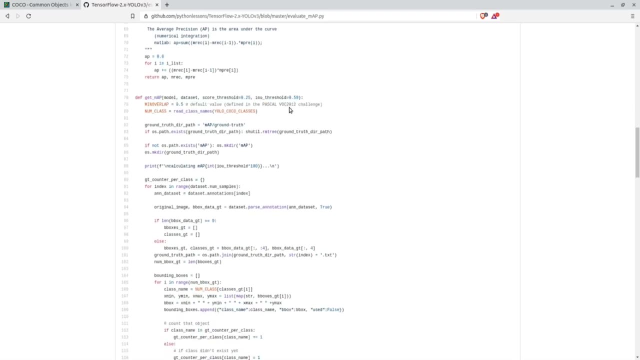 And now I will explain the evaluation process in a few sentences. The whole evaluation process can be divided into three parts, Of course, and I'll open this my script. So we call this script and, as you can see, there is default values. 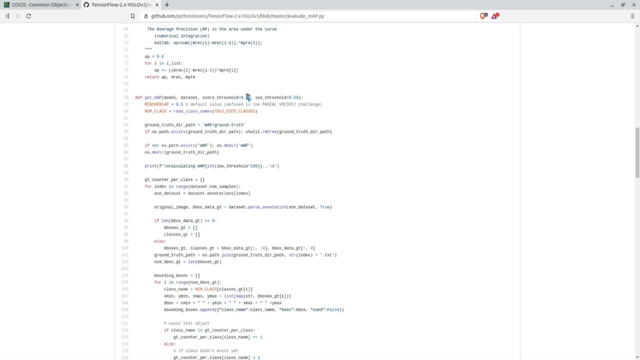 There is our IOU threshold and score threshold. As default, I'll use 0.25. And here is minimum overlap, which is from Pascal was 2012.. So here at first, it creates a map folder in our local directory. 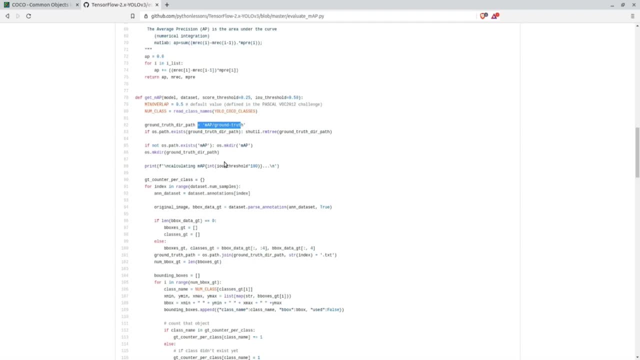 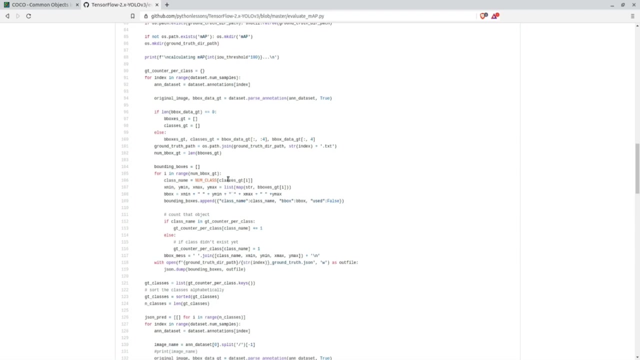 And in this folder we create a ground truth folder and where we create a JSON file for every ground truth image bounding box. As I said, this will be short. In the second part, most part is done by our YOLOv3 model. 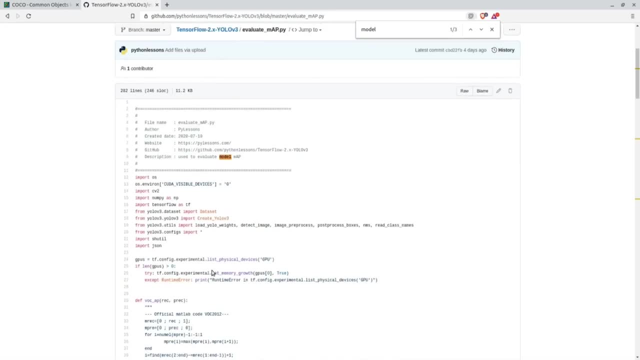 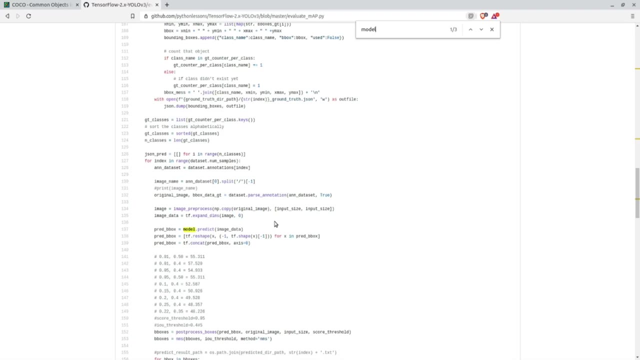 I can. Where is our model? I can write search, So here, And it runs prediction on every image. similar way, as in the first part, It creates JSON files for every class We have and puts the detection bounding box accordingly. And in the third part, 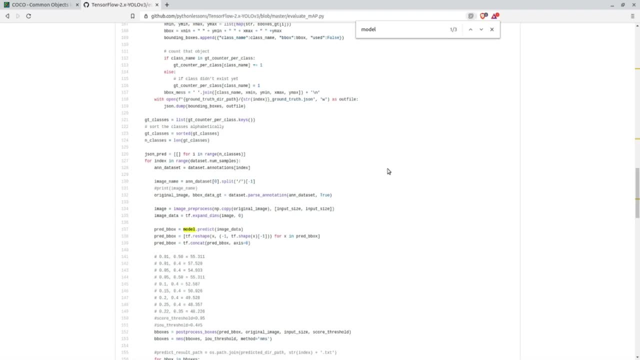 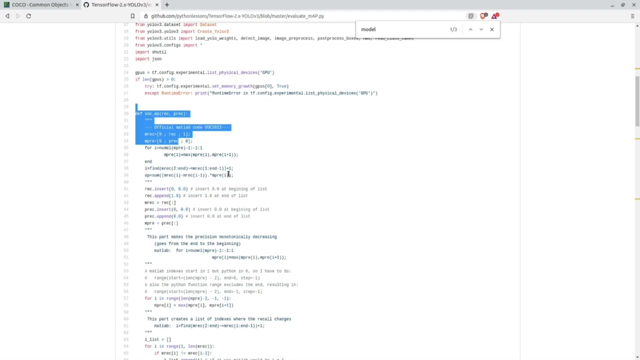 we already have detected ground truth bounding boxes. I mean detected and ground truth bounding boxes. So what is left to calculate the map? So, for each class, with a what's AP function, which is here. So, after we're calculating the average precision, 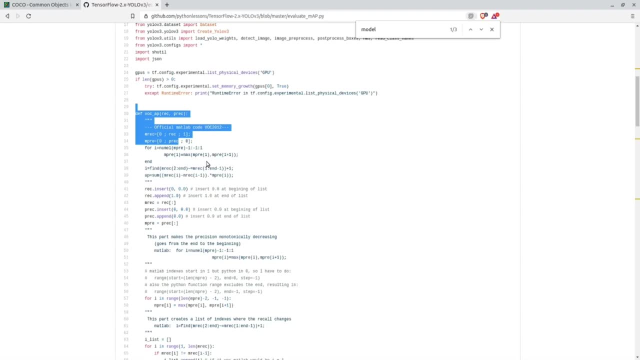 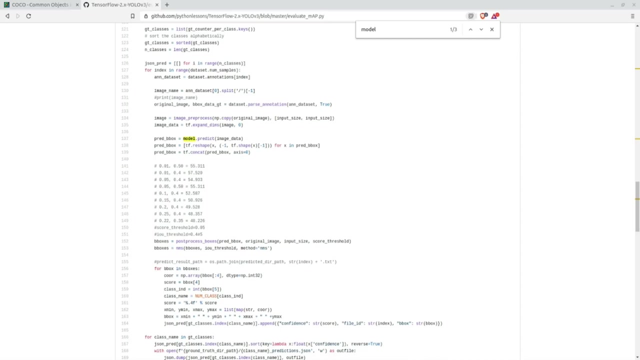 for each class, we have results of them And what is left is we need to average it and we will receive the map. That's quite simple And, of course, if you would like, I can run an example for you. So I will open my directory. 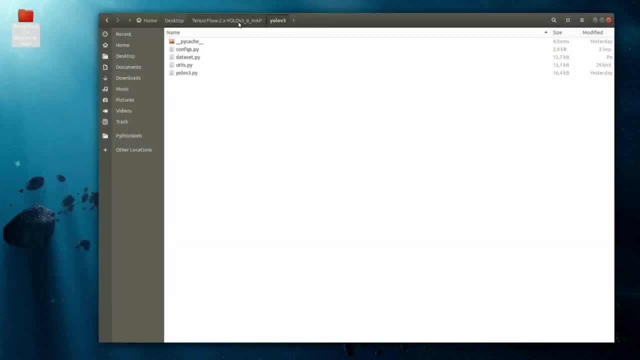 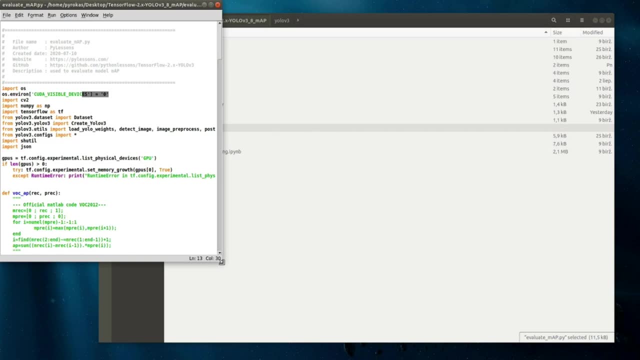 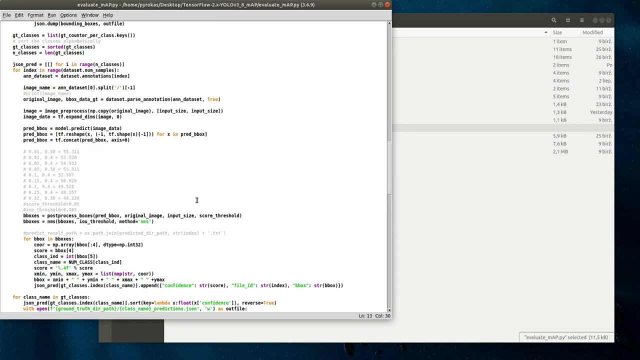 And, of course, I will open my evaluation map function. It will run on my first GPU, So OK. So OK, Here I was running it for I don't know a lot of times and checking the results, how they change. 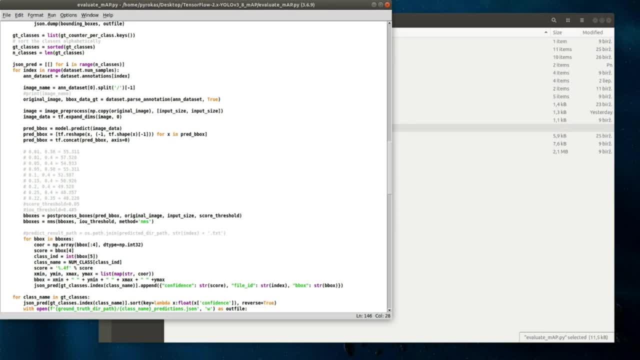 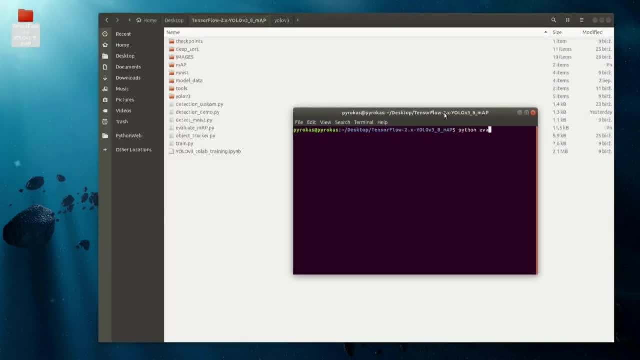 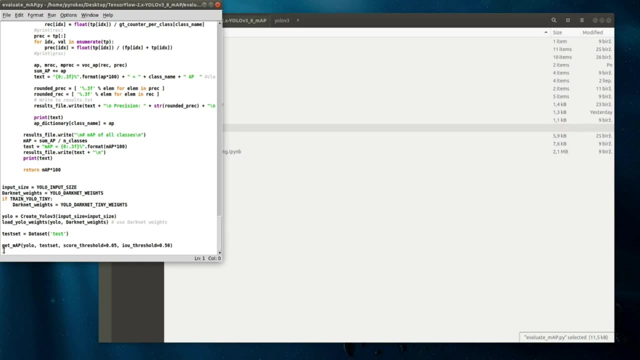 depending on threshold and IOU. And right now I can open terminal and just write python evaluate map And as you can see, let's see, Right now it will run a map with threshold 0.05 and IOU of 0.50. 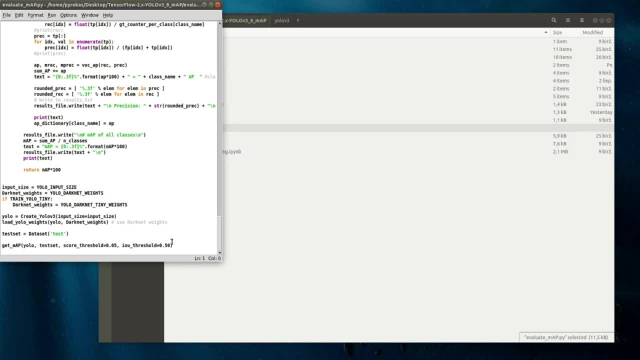 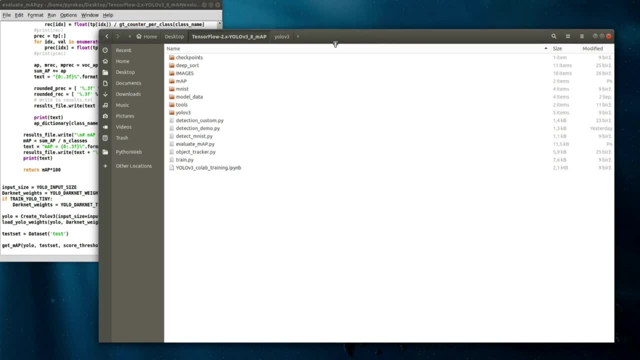 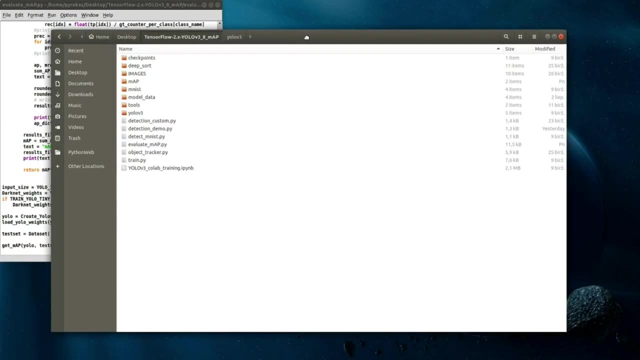 And, of course, I think that I will implement this function into the train by function that when we finish training, it by default gonna call this function to evaluate our map of our model. So that's it. I can run this now. 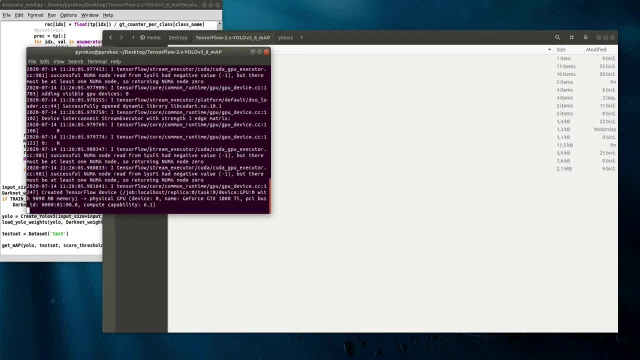 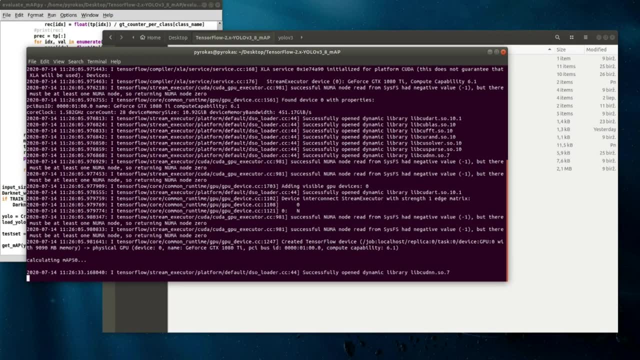 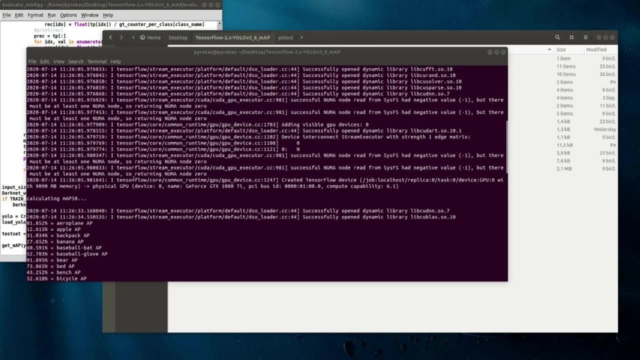 And it will take a while, So I'll just wait and come back when it finishes. So I'm back And, as you can see there, we have our results here And it finished to measuring the mean average precision, As you can see. 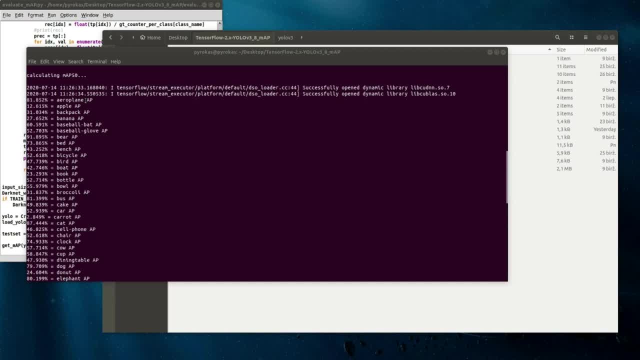 it measured average precision for every class And, as you can see, for example, airplane is 81%, backpack 31%, banana 27%, baseball bat AP is 60%, and so on. This is it, So we have 80 COCO classes. 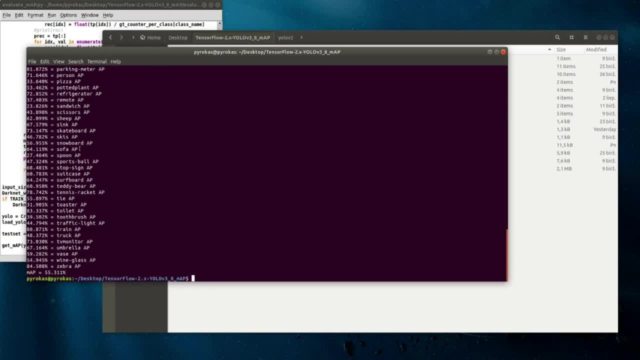 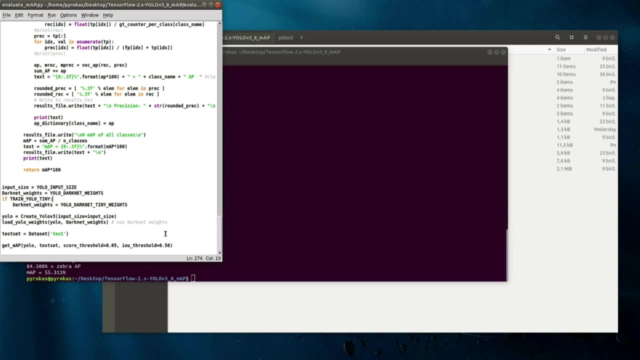 which is used here. So actually these all classes are simply averaged And, as you can see, it receives 55 mean average precision. But keep in mind this is only with a threshold of 0.05.. And to be: 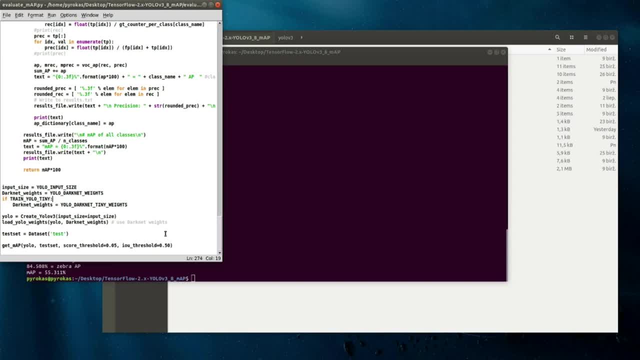 It's not recommended by me. I recommend you to use some kind of precision of 0.25 or even 0.5 in your real-time custom model, and so on. But it is what it is And, as you can see, 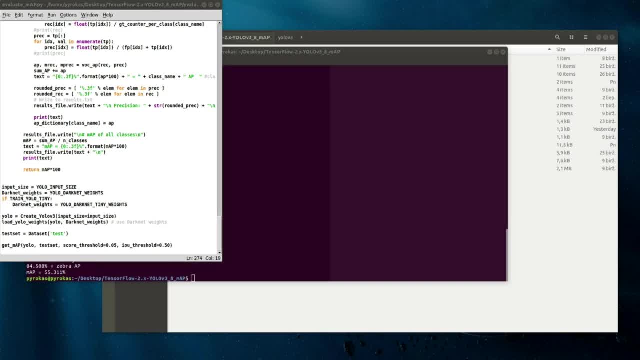 we achieved quite similar results as we had As it was published by real YOLO3 paper And I can say that My Scripts kinda works. So that's it for this tutorial part, And I did this tutorial because it's valuable to know how to calculate. 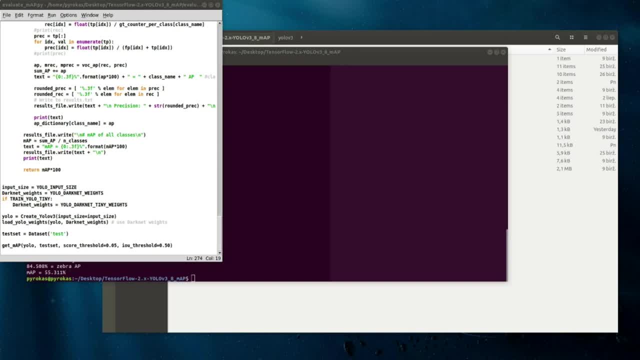 the mean average precision of our model. You can use this metric to check how accurate is your custom training model. with validation dataset. You can check how map changes when you add more images to your dataset, change threshold or intersection over the union parameter. This mean average precision. 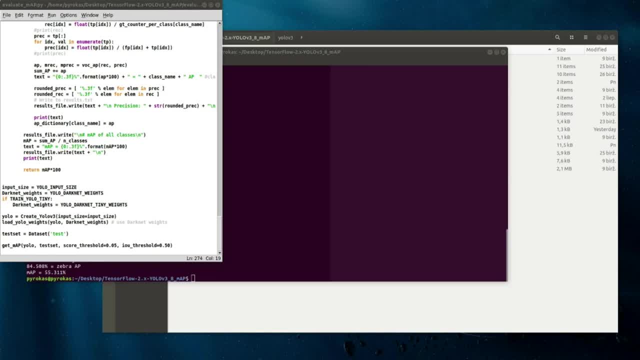 is mostly used when you want to squeeze as much as possible for a custom model. I thought about implementing map into the training process to track it on tensor board, but I couldn't find an effective way to do that. So if someone finds a way,